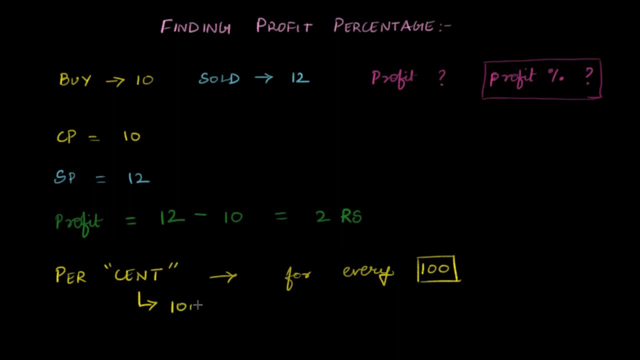 centimeter. you know that always has something to do with hundred in it. so in general, what does a percentage mean? let me just bring it all up over here. so percent in general means per hundred. so a simple way to say what a percent is is the numerator. it's the numerator of a fraction. 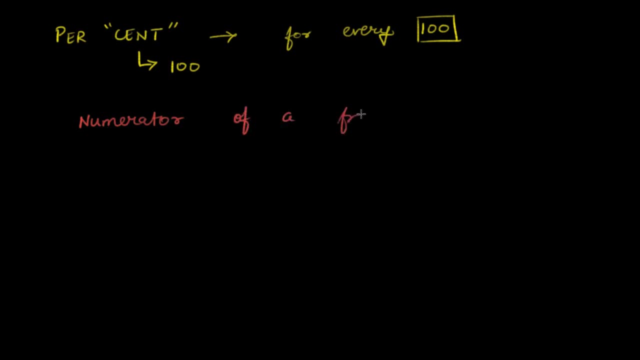 whose denominator is hundred. numerator of a fraction whose denominator whose denominator is hundred. i know it's a big way to say it is hundred, but this big sentence in the language of math is simply something by hundred, something by hundred. if this is 30 by hundred, then we say: 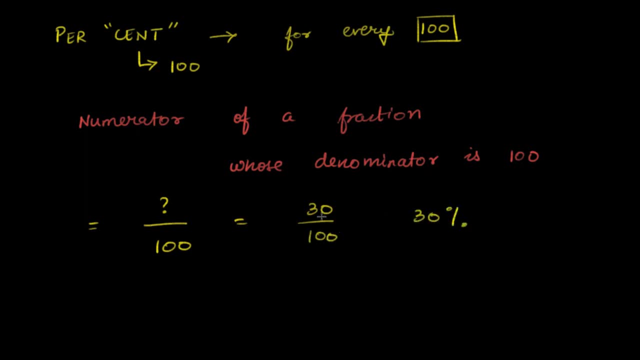 this is 30 percentage. these two sentences are the same thing. 30 out of 100 and 30 percentage are exactly the same thing things, just two different ways to say the same thing, and you probably know this, but i'm just using a refresh that we can now look at what profit percentage means. so this had been 15 by 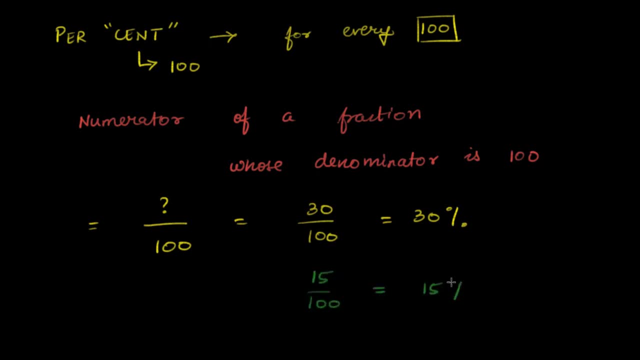 hundred. that's another way of saying 15 percent. in fact, this number can be more than 100. it doesn't always have to be less than 100. i can have 120 by 100. and what is that equal to? that's 120 percentage. now let's get to the question over here, which is not just the percent, but what's the profit percent? 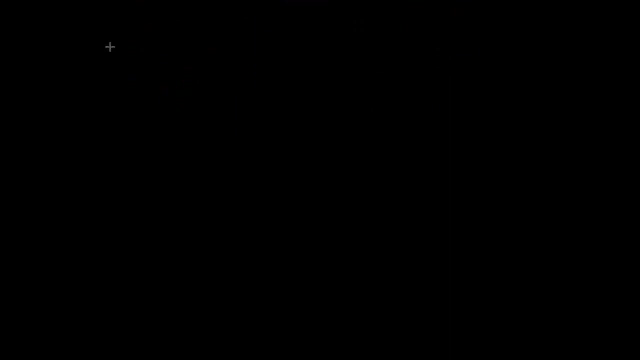 so let's, let's do that over here. so the question wants you to find out the profit percentage. i'm going to write this out like this: profit per hundred cost price. that's what this sentence actually means. so when we say: can you calculate profit percentage when your cost price was what was it? again, it was 10, and 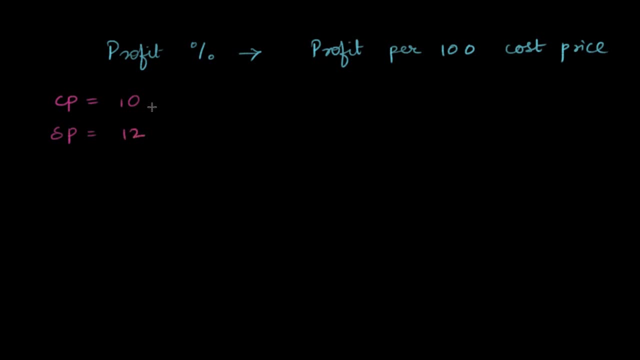 your selling price was 12. when it's asking you: can you find profit percentage? what do you really being asked is: can you find the profit per 100 cost price? another way to say the same thing is profit for a cost price of 100. cost price of 100, and this will become more clear with. 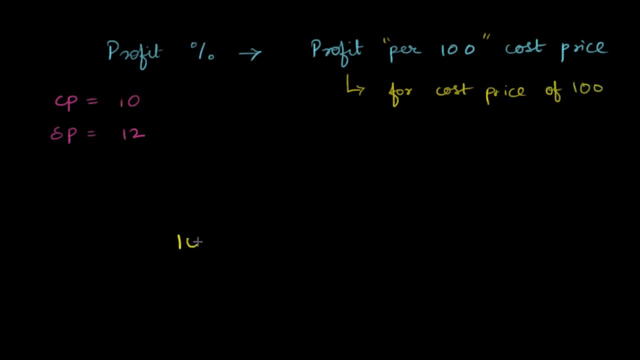 an example. so cost price was 10. how much did you make? two rupees? and now what is it asking? this question is asking what profit would you have made if your cost price was 100 rupees? so you bought for 10 rupees. let's write the cost price over here: you bought for 10. 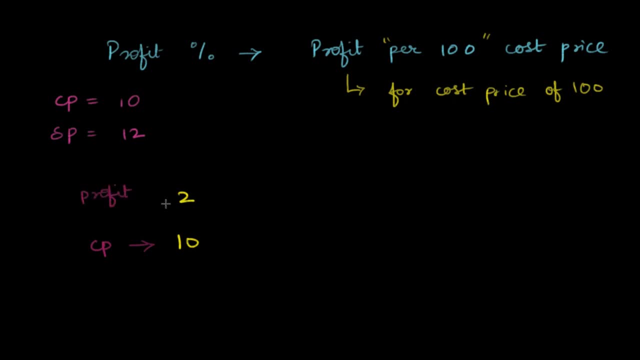 and you made 2 rupees, so profit is 2 rupees. what if you had bought for a hundred? then how much would your profit have been? if you calculate this answer, this is what we call profit percentage. and now there are many ways to get to this answer. now, one way that I think: 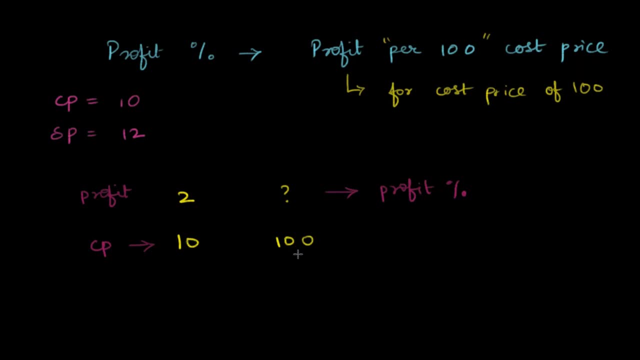 about. it is for you give me- you gave me 10 rupees. I made 2 rupees profit. if you give me 100 rupees, how much will I make? so this is very similar to asking the question: 10 bananas cost 2 rupees, then how much will 100 bananas cost? we have solved many problems. 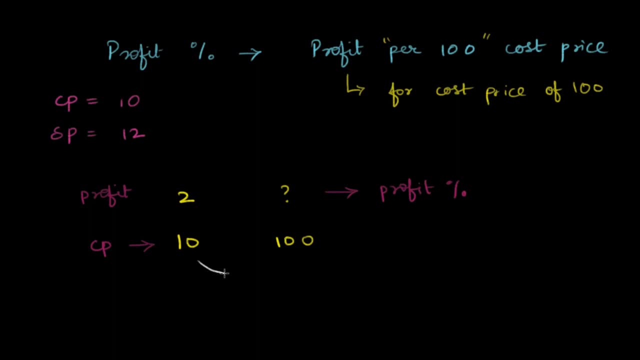 like this. so in my mind I'm just going: ok, 10 times 10 gives me 100, then 2 times 10 will give me what? because I know how to multiply by 10 to go from 10 to 100. so then I must. 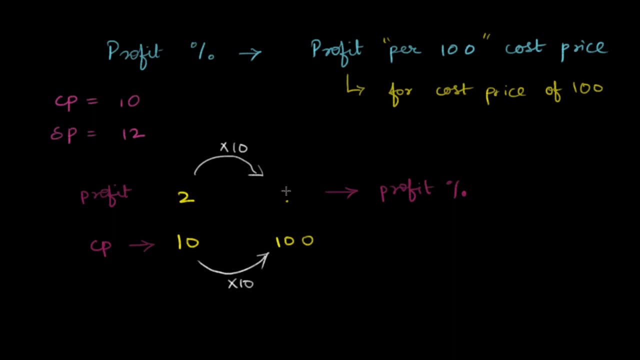 multiply 2 with the same thing to get to the answer over here. and so what is that answer going to be? 2 times 10 is 20. so 20% is the answer to the question is 10 times 2 is 2, this question that we have. So for 10 rupees cost price, I made a 2 rupee profit, So for 100 rupee. 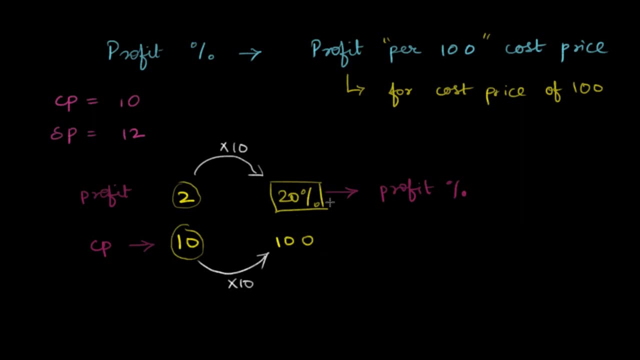 cost price, I'll make a 20 rupees profit, Or in other words, I have a 20% profit. Now notice that this is not a new thing you're learning. Another way to look at the same thing is as a fraction. 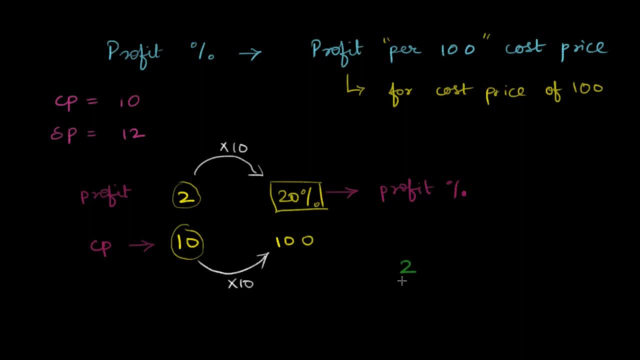 problem. So this is the same thing as asking: you made 2 rupees for 10 rupees. How much will you make? How much will you make for 100 rupees? Now, isn't this just a fraction problem where three? 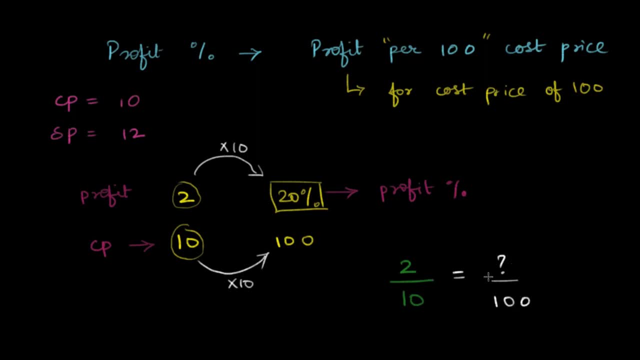 things are given and you have to find this thing over here. There are many ways to do it. We just did it in one way, by asking to go from here to here. 10 has been multiplied by 10.. So if this fraction has to be equal, you have to multiply this also by 10.. And that's what we did. We wrote. 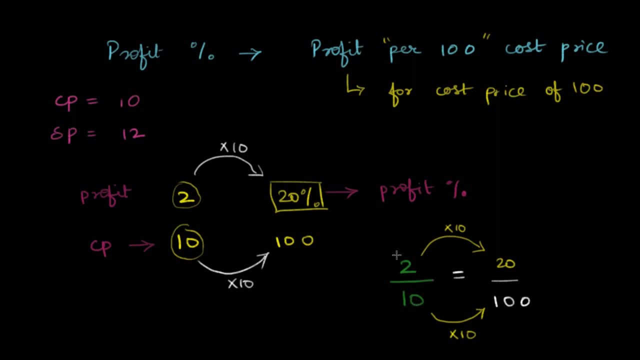 20 by 100.. So the question is asking you: convert this fraction to a fraction whose denominator is 100. And you'll notice that you have to multiply this by 10.. So you have to multiply this by 10.. You don't need any formula to do this. One of the problems that I see is that students tend to 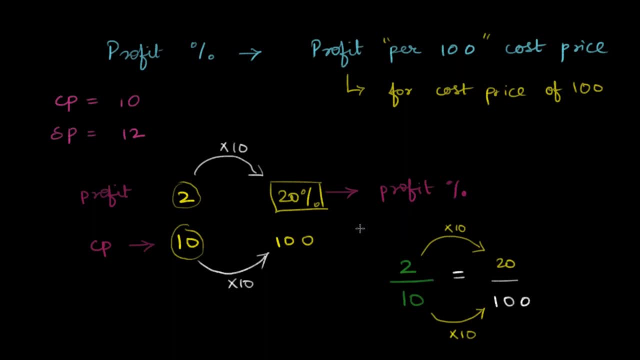 think that profit and loss has some formulas, and then simple interest has other formulas, Discount has other formulas, but you'll start seeing that all of these are the same problem. Let's look at one more problem to see that Maybe this time the cost price is 1000.. So you're buying a big thing. 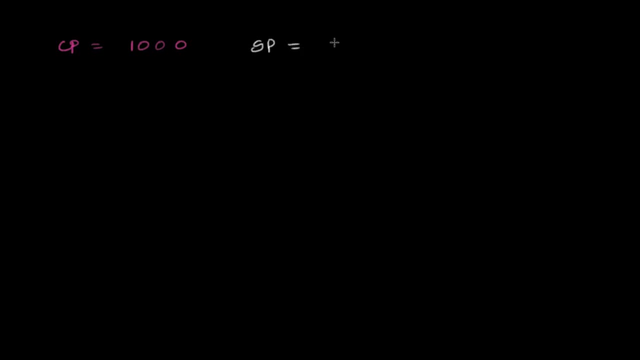 now And then you're selling it. You're selling price is 1050.. So how much profit did you make here? Now, the profit you made is 50.. Rupees 1050 minus 1000.. So you made a 50 rupee profit bigger than what the previous person made. 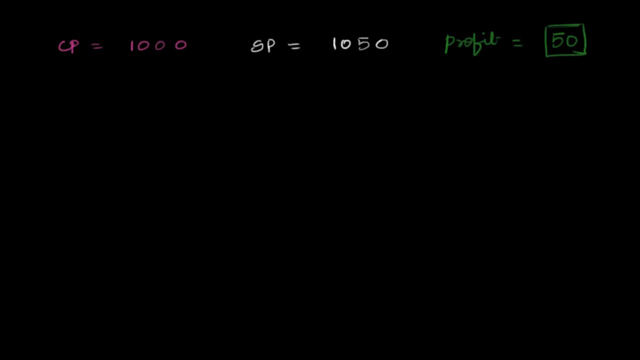 He just made a 2 rupee profit, But let's see what the profit percentage is. Profit percentage: What is that going to be? Now, you know everything you need to know to calculate the answer to this question. So pause the video and look at what answer you get, And let's let's think this through. 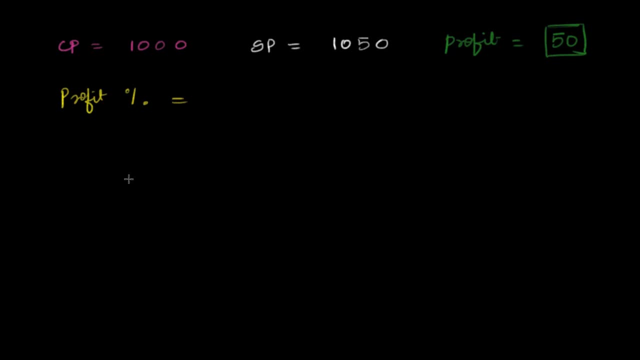 together. So you've thought, and you have an answer with you, Let's do this together. The way I'm doing it in my head is: I'm going: okay, So the cost price was 1000.. The cost price was 1000. And the profit I made was 50. And when 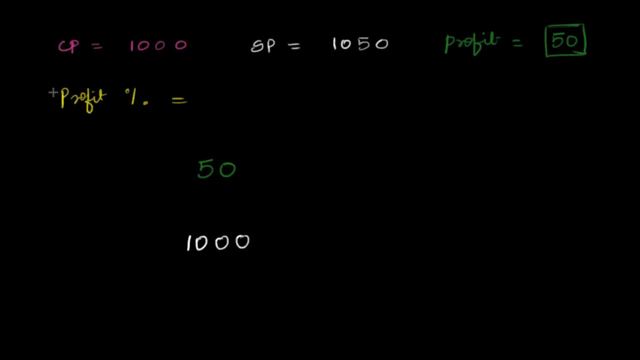 somebody is asking me what profit percentage is. in my head I am breaking this down into: oh, you want profit percentage. In other words, you want: how much profit would I have made if my cost price had just been 100?? And now I look at this and I go: okay, 1000 rupees. I made 50 profit for 100. 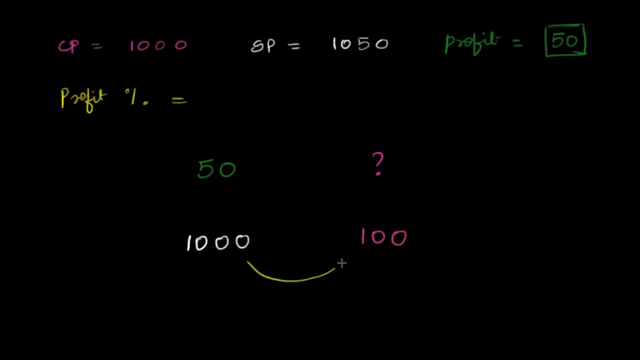 rupees, how much would I have made 100.. I have to divide by 10, or in other words multiply with 1 by 10.. 1000 by 10 gives me 100.. So to keep the whole thing equal, I have to multiply this also by 1 by 10.. And what will I get over? 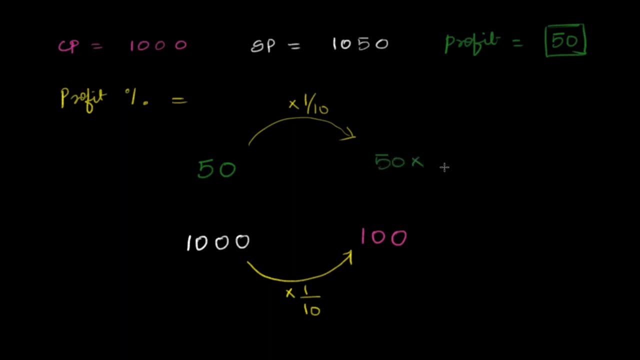 here 50 times 1 by 10.. 1 by 10.. Or in other words, 5%. 50 by 10,, 5%. So the profit percentage here is 5%. Notice that this is nothing different. You've just been asked this fraction, question 50 by.